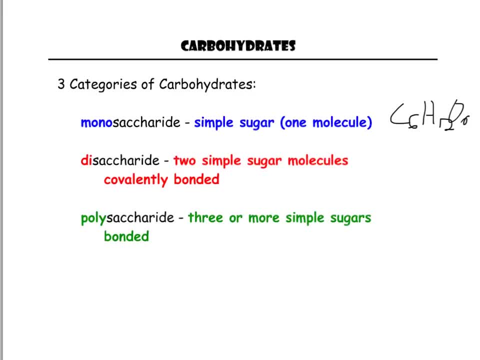 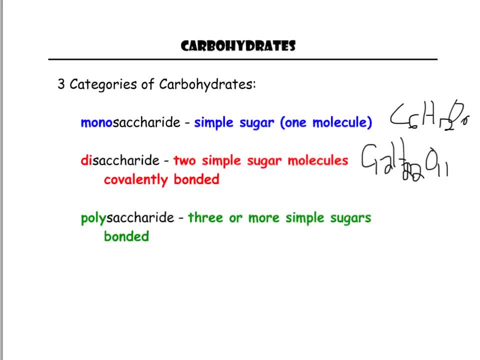 And you'll notice here, this one here is C12H22O11.. And you'll notice here, this one here is C12H22O11.. And the second one no longer follows this pattern of twice the hydrogens and the same amount. 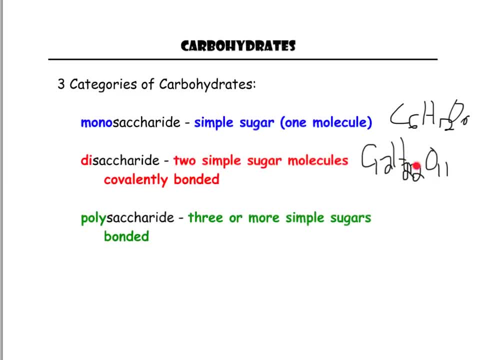 of oxygen. So we went from 12 carbons but now we only have 22 hydrogens and we only have 11 oxygen, And we'll look at why that is on the next slide. And then our last form is going to be a polysaccharide. 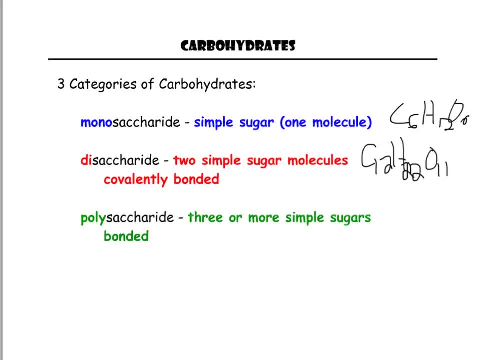 Again, we've seen poly before. Poly meaning many, and that is when you have three or more simple sugars bonded together. There isn't going to be a set chemical formula for this. this, like we've seen with you know the monosaccharide or disaccharide, and that's because 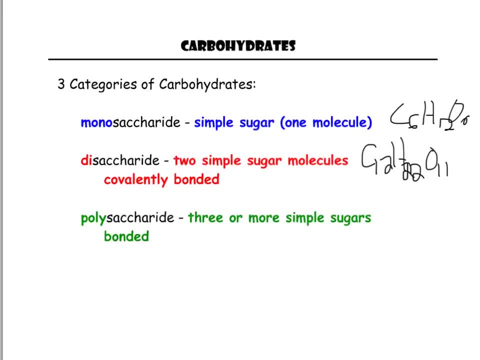 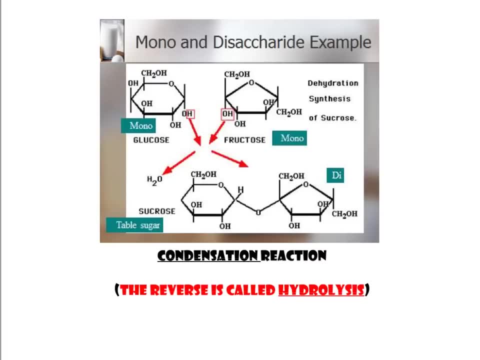 poly is going to depend on how many sugars were bonded to one another, and here we look at how a monosaccharide and disaccharide are related. so a monosaccharide is going to be one of these simple sugars. here again, this is basically just a cyclohexane ring. it's just looked at from an 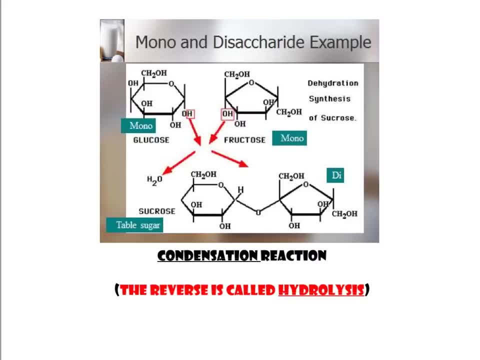 angle, and then it has a lot of different alcohol groups on there, but that's an example of what a sugar is. and then what happens is when two monosaccharides join together. this is actually an example of our condensation reaction that we learned about, so you'll notice that the one 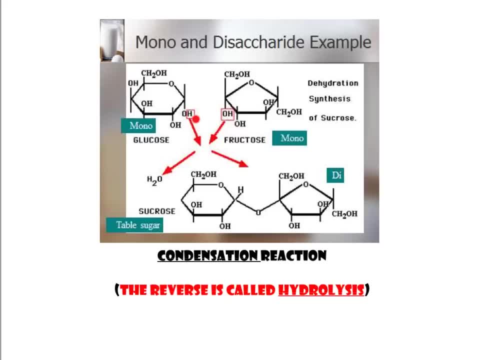 hydrogen here and the oh from here are going to break off and we get this h2o again and then we are going to have our disaccharide. so that is now two sugar molecules combined and you'll notice, before when we talked about our monosaccharide, it had a chemical formula. 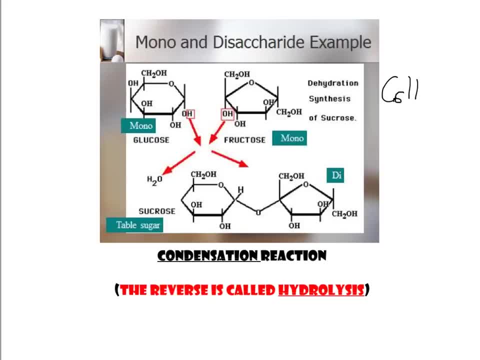 or a molecular formula of c6- h12- o6, and then the disaccharide was c12- h22- o11, and if you look at these, you'll notice that this disaccharide here has just lost this water, and so that's the. 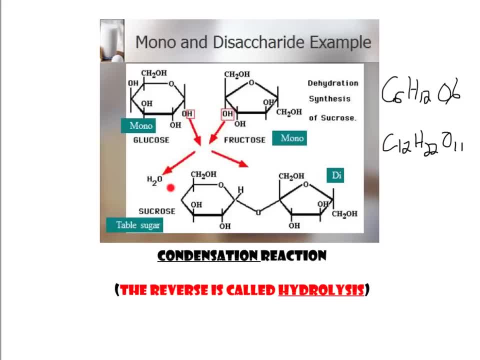 difference between these two? they're number of carbons didn't change, but this water comes off, and so that's why, instead of being c12, h24, o12, this has just lost this water molecule over here, and that is why it's still called a condensation reaction. the reverse of this, however, is if we started with the disaccharide and we 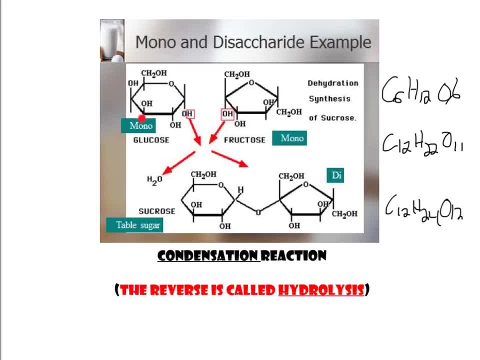 added water into it. you can actually split that apart and get a two monosaccharides. the reverse of a condensation reaction is going to be the disaccharide, and the disaccharide is going to be called hydrolysis. and really quick, here's an example of a polysaccharide, again poly meaning. 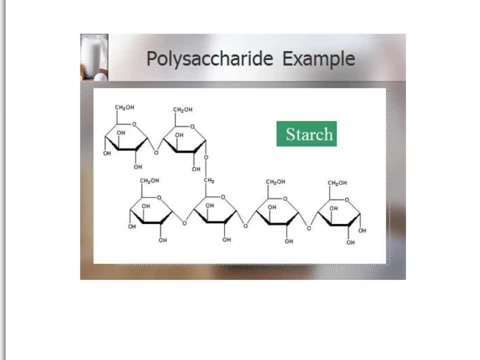 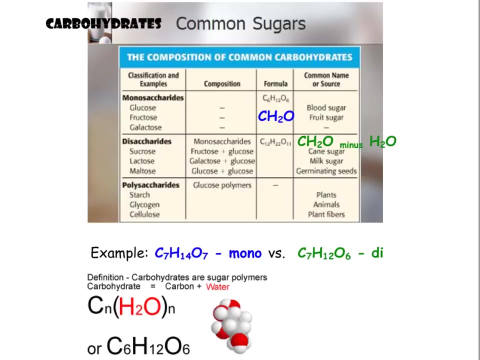 many saccharides, so many sugars joined, and here we have one, two, three, four, five, six sugars joined together, and this is actually an example of starch. so far we have talked about mono, di and polysaccharides. so one thing i do want to point out is that a disaccharide is not necessarily two monosaccharides joined together. 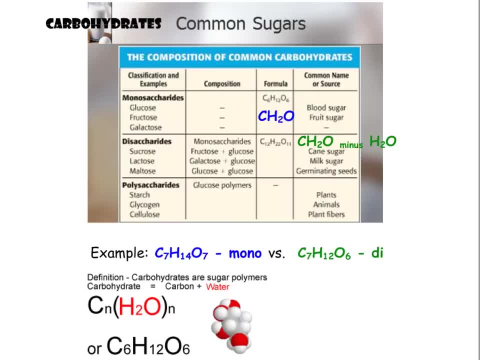 the way that it works is. a disaccharide is something that follows the generic formula of cx, h2x, ox, and then you subtract an h2o off of it. so let's look at an example down here. if we have c7, h14, o7, that would be a monosaccharide. 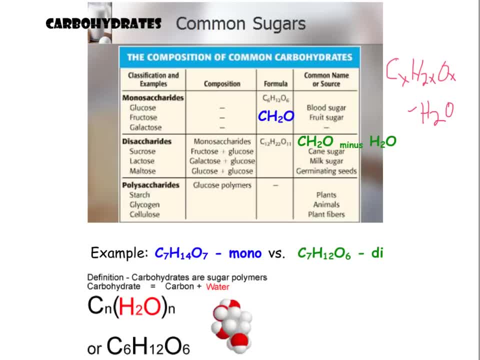 and the reason this is a monosaccharide is because it follows this generic formula where we have cx, so c7, h2x, so h14 and then o7, so we have that 7 there again. now the disaccharide version of that is: if we took this and we subtracted h2o off of there, you'll notice. 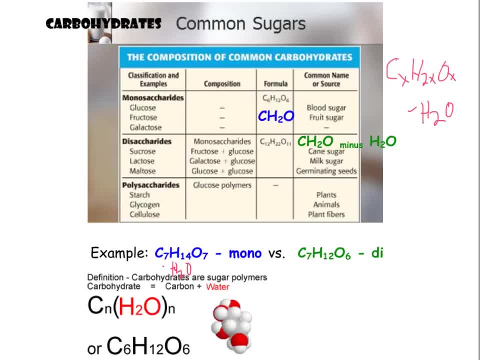 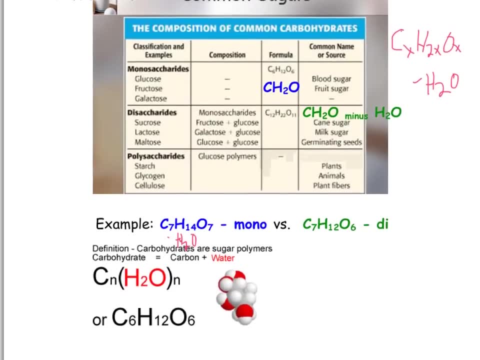 we get this disaccharide which is c7, h12, o6 and then a generic definition of carbonyl. so what we found on our formula of disaccharide is that disaccharides have 3 types of carbohydrates. the first one is, i said before- is these polymers are polymers and so we need a 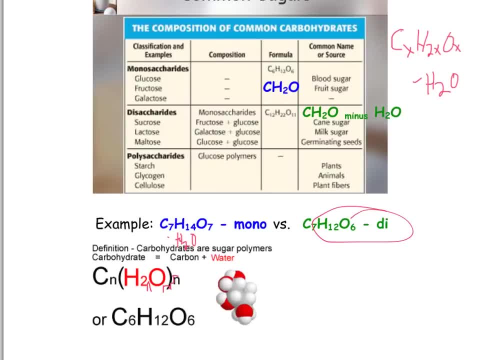 misnomer. and then I made this formula to be able to make these polymers the same way. if you had any other kinds of polymers, then you would be able to make these polymers the same way. next, we have a formula of carbolytes, the carbolytes that are water-based or something. 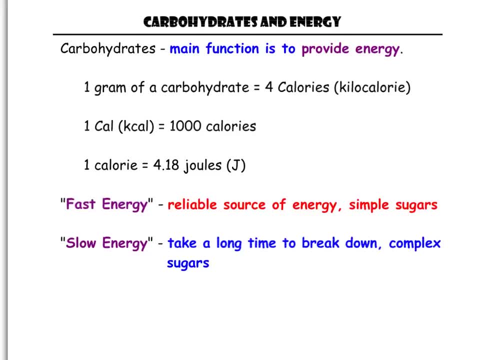 that is carbolytes is that they are sugar polymers or you know some sort of carbohydrate. If you've ever heard of somebody who's going to run, say, a marathon or some sort of race, they will often carbo-load, And that is because carbohydrates provide us a lot of energy. 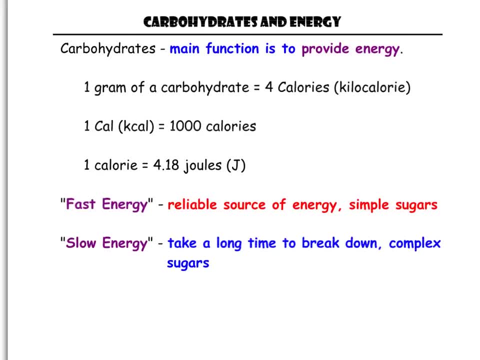 And the way that they do that is so fast. energy is something that is a reliable source of energy, And those are like your simple sugars, So if you get a candy bar or something like that, you get energy very, very quickly. Slow energy are something that takes time to break down. 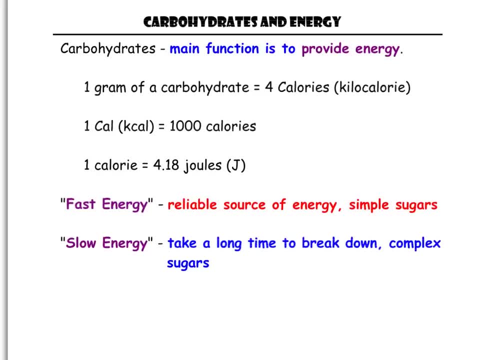 Those are going to be your complex sugars or your complex carbohydrates. So a good example of that would be: like your pasta And that's what a lot of runners will carbo-load on, because that will slowly release the energy, because they are very, very, very long carbohydrate chains. 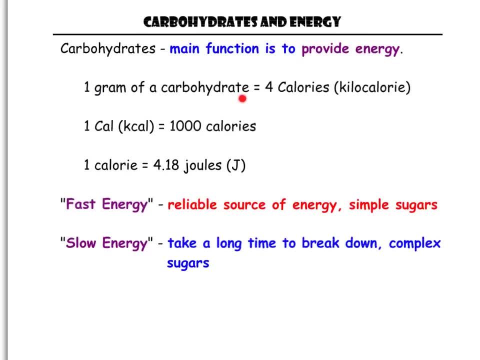 One thing to know with carbohydrates is: one gram of a carbohydrate is equal to four calories. Now, key thing with calories here is that we have this capital C, Because it actually is going to be. I know it's a really confusing way to do this, but four calories with capital C is actually equal to 4,000 calories with a lowercase c. 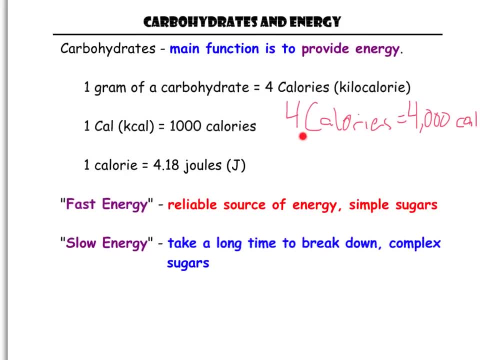 So we have to be very careful with that. this unit that whenever we look at a food, it will always be talking about this capital C. So if you look at food and it said it had four calories in it, that is actually 4,000 calories. 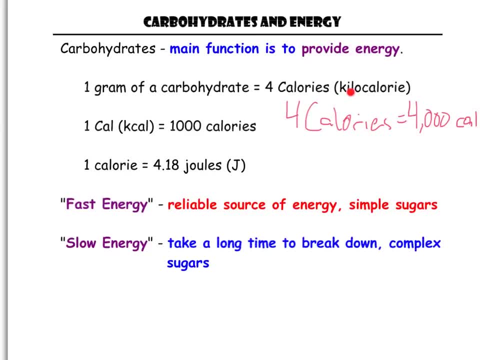 Because it's capital C Technically stands for kilocalorie, And that's what this is talking about. down here is one capital C calorie is equal to 1,000 kilocalorie, Or is equal to a kilocalorie which is 1,000 calories. 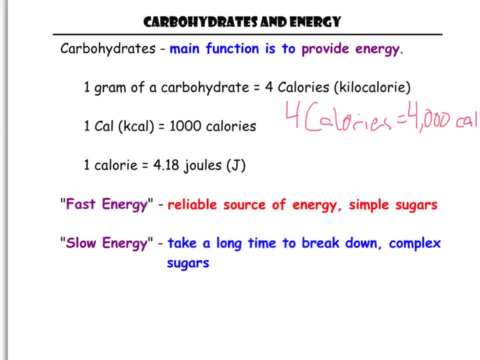 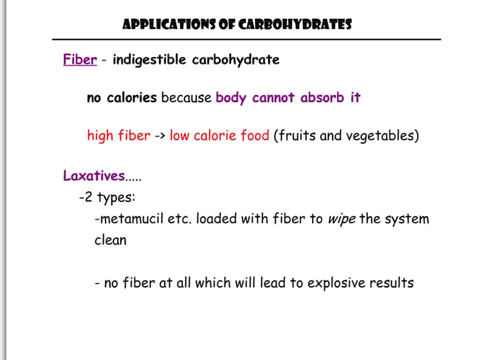 And then one calorie lowercase c is equal to 4.18 joules of energy. So a lot of us have heard about fibers. Fibers are basically just indigestible carbohydrates, And the reason for that is the body can't absorb it. 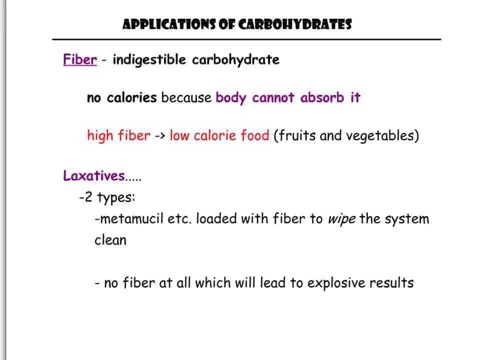 So a lot of your fibers actually don't have any calories because they're indigestible. Your body doesn't have a way to break that down, So therefore they provide no calories because they're basically just going to pass through you. Something that has high fiber is going to be a low-calorie food, so your fruits and your vegetables. 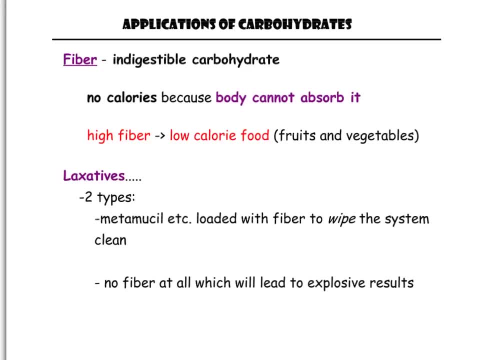 And a lot of us have heard of that. If you're ever a constipator or anything, you need to eat a lot of fiber in your diet Because it's just going to Basically pass right through you. And then laxatives are the more common term that we've heard of with, we'll say, helping to clear you out. 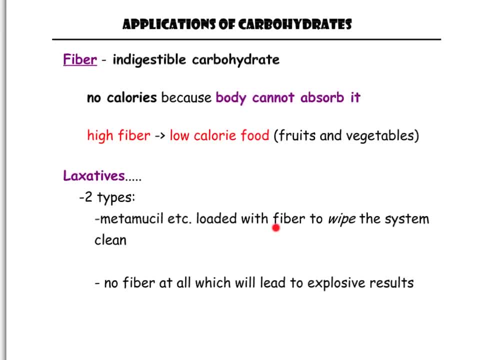 So two different types of those. There's metamucil, which is loaded. They just have tons and tons and tons of fiber which help to wipe the system clean, And no fiber at all, which, well, that can lead to explosive results. 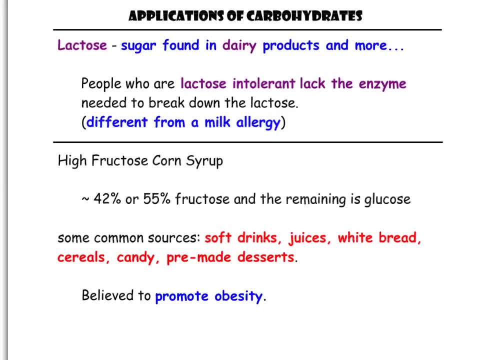 So another application of carbohydrates is lactose. Lactose is sugar that is commonly found in dairy. It's found in dairy products and a lot more. So if you've ever heard of somebody who is lactose-intolerant, what that means is they're lacking, basically, the lactose enzyme. 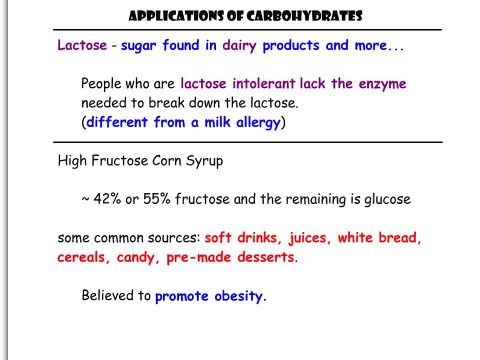 And you can think of an enzyme as kind of like the key. so it's what knows how to break apart those lactose sugar molecules. So if somebody is lactose-intolerant, they're lacking this enzyme that knows how to break apart the sugar molecule that is found in milk. 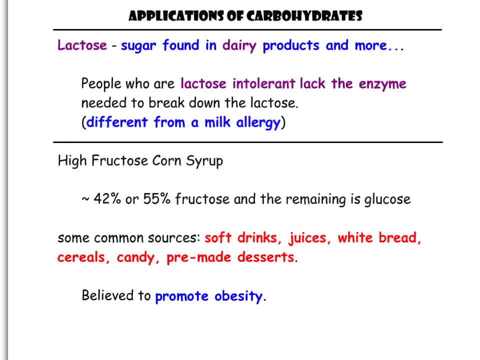 And then there's also what's called high-fructose corn syrup: Forty-two or fifty-five percent of fructose and the remaining is glucose. So high-fructose corn syrup just means there's a lot of the fructose sugar in there, And common source of this are your soft drinks, juices, white bread, so on. 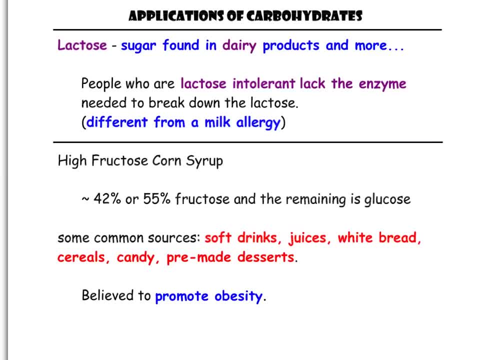 And they're believed to promote obesity because, again, they are not dissolved all that well by the body, So the body's not going to know how to break those apart. They're not going to leave you And your body is just eventually going to turn them into fat as a way to store that energy. 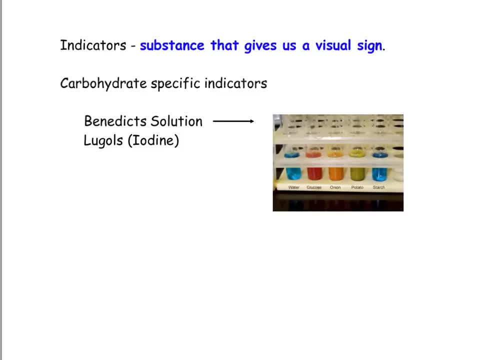 Tomorrow we'll be starting our lab on carbohydrates, So the way that we're going to do that is we're going to use what's called an indicator, And the indicator you've worked with before is when we did the titration lab, And that's where you added a couple drops of this.